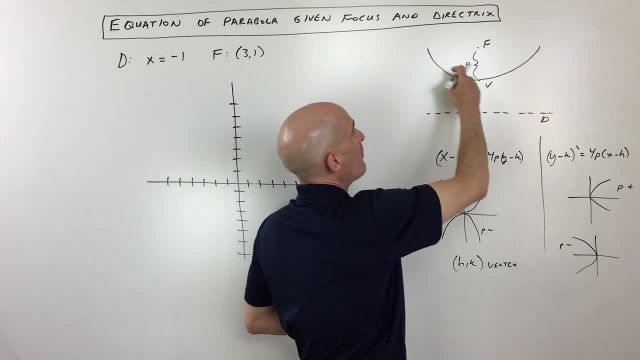 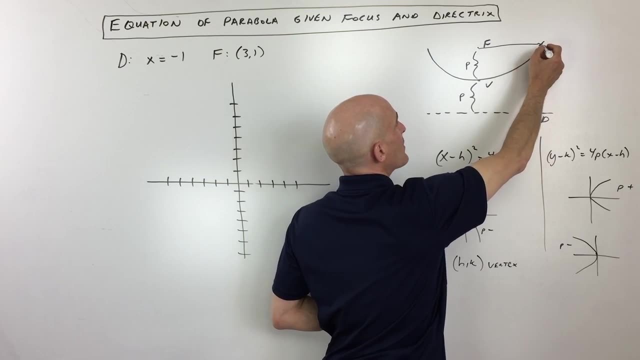 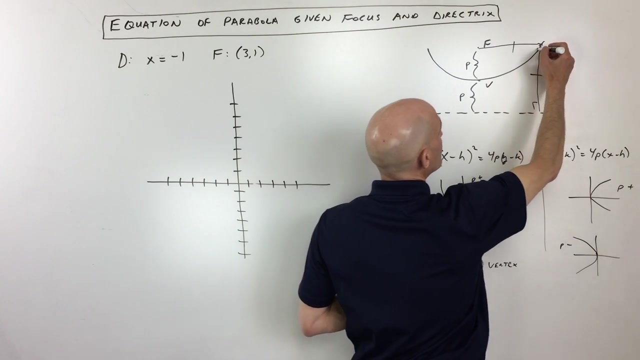 What basically is a parabola? Well, a parabola is the set of all points, okay, such that if you pick a point on that parabola and you measure the distance to the focus and you measure the distance to a line called the directrix, those distances are always going to be the same. So the idea is, if you were to go further out on this parabola here, you can see the distance to that focus is getting longer, but so is that perpendicular distance to the directrix is also getting longer. But those points on the parabola, this U-shaped graph, okay that. 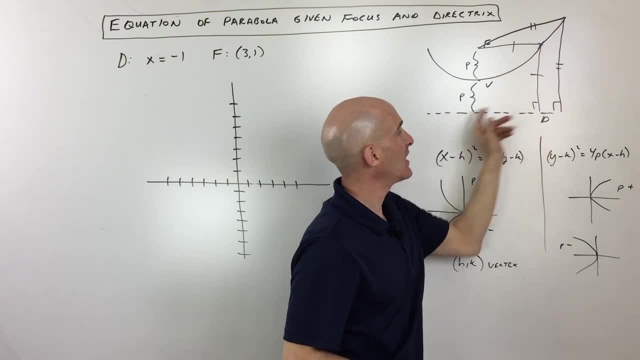 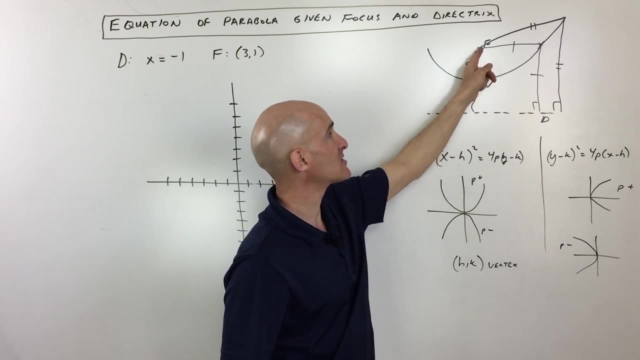 are always going to be equidistant from a given point, called the focus, and a given line, called the directrix. The other component of parabola is this distance between the vertex and the directrix and the vertex and the focus. We call that distance p, and the basic equation of a parabola is in the 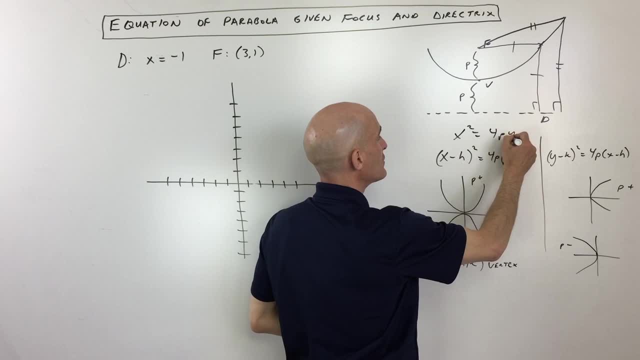 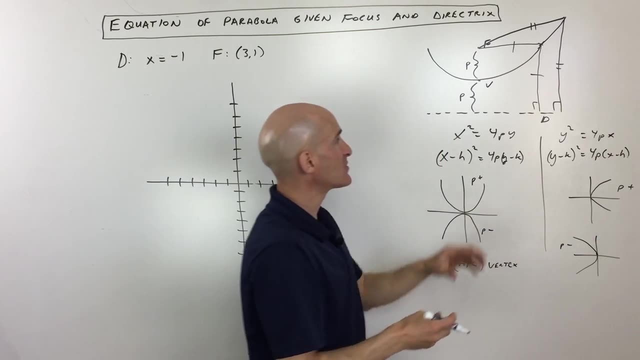 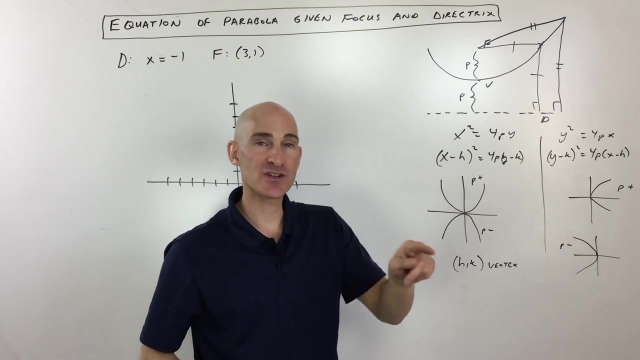 form: x squared equals 4py or y squared equals 4px. Now, the thing to realize is that you know, these parabolas can be picked up and shifted left and right, up and down, The way I've written the equation here. this is where the vertex, or that bending point, that turning point, is at the origin. 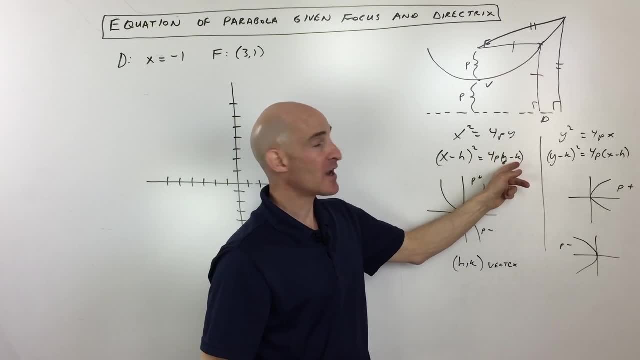 but you know, you can see the h and k, can shift the graph left and right, up and down, but the key thing to remember is that if the x term is squared, that means the parabola is going to be opening either up or down. if the p is positive, it's opening up. if the p is negative, it's opening down. 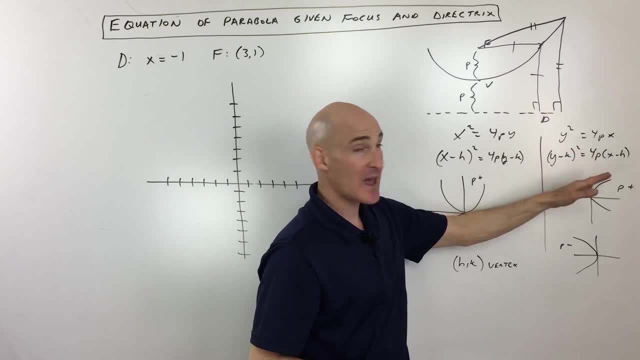 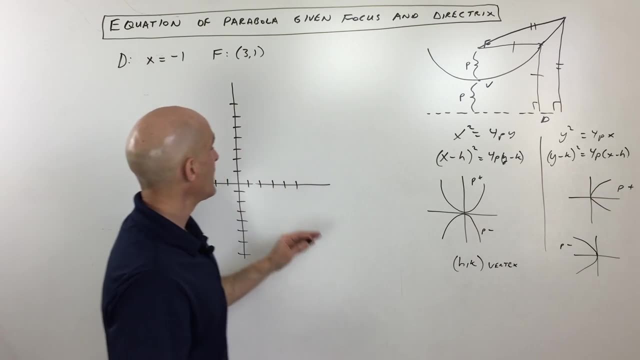 and then for the y squared. if you have a y squared term but not an x squared term, that means it's opening to the right or the left, left if p is negative, right if p is positive. so let's get into this problem and see if we can graph it and write the equation. so the directrix here is: at x equals. 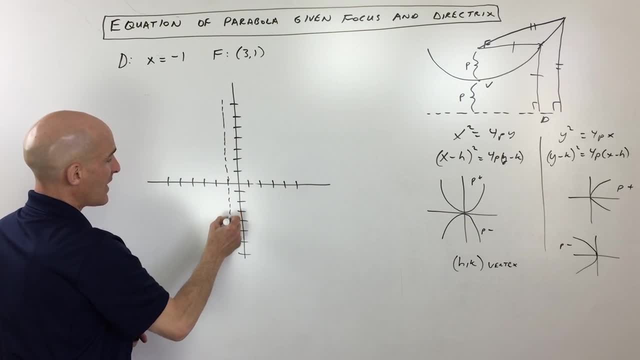 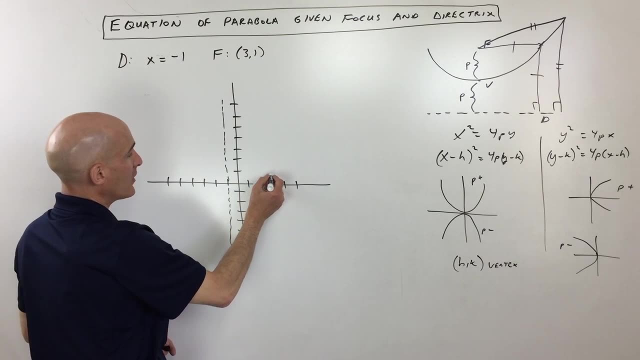 negative one. so let's go ahead and sketch that in. so that's just an imaginary, you know, invisible line, okay, and we'll just write that x equals negative one, right there. and then the focus is at three one, which is right there. i'll just label that the focus. now, the thing to realize is that. 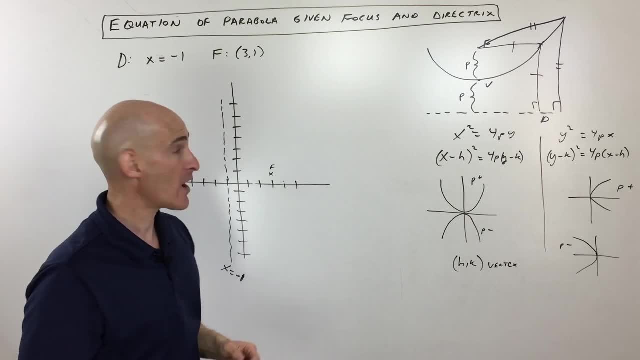 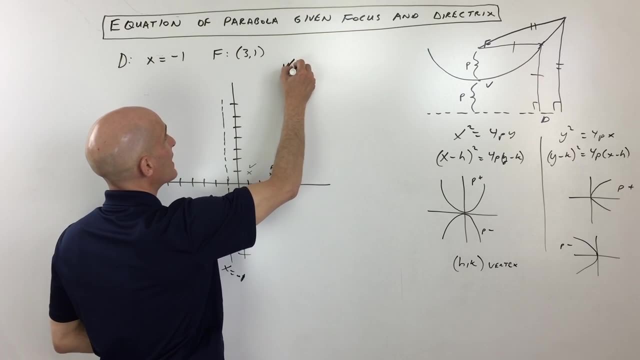 the vertex is halfway in between the focus and the directrix. so if we find that midpoint, you can see that's going to be right here at you, one one. so let me just write that down. the vertex is at right: one up, one. okay, so now the distance.